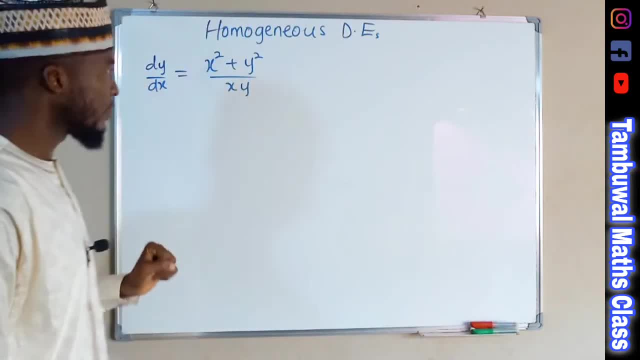 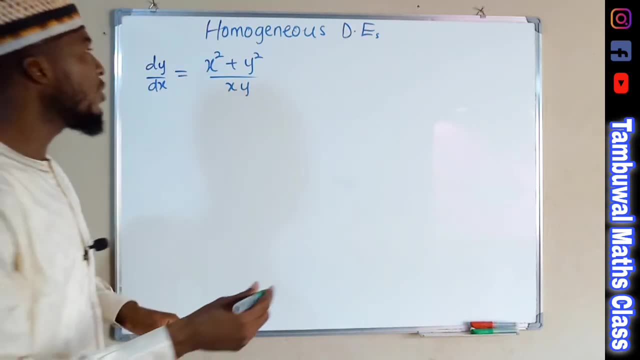 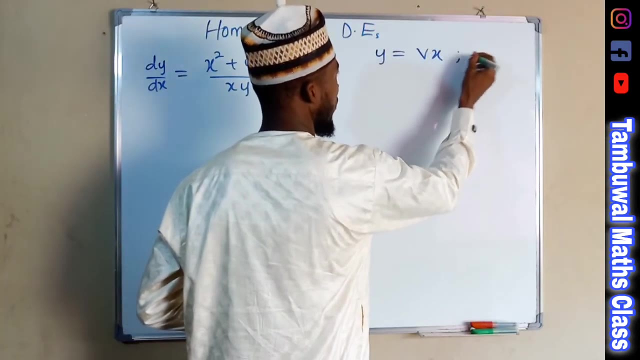 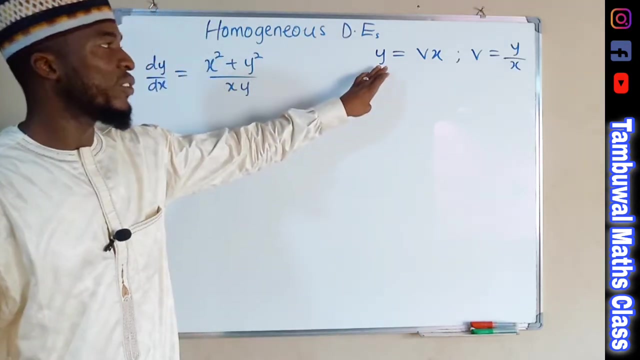 So let us now look on to this form. This is a homogeneous differential equation which you cannot separate the variables. So we are going to replace y with vx, such that this v is equal to y over x. Now we are going to differentiate y with respect to x, dy over dx. 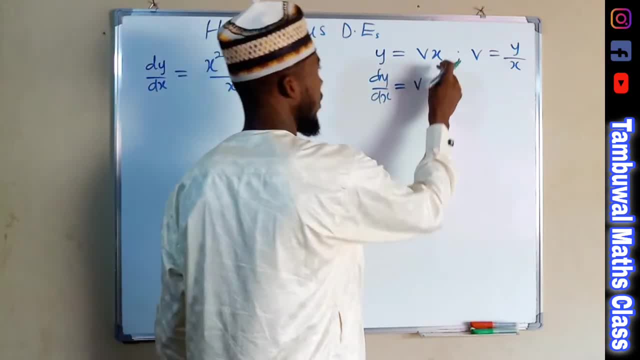 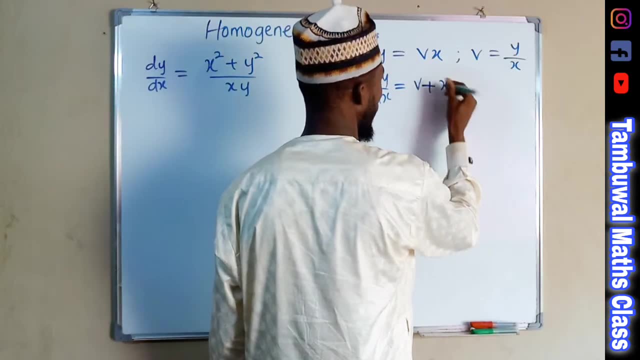 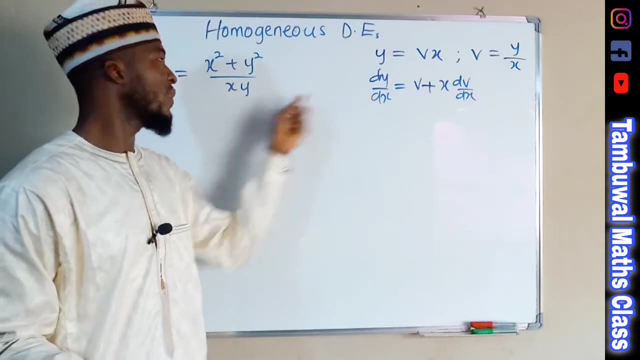 Using product rule, you keep the first time constant. If you differentiate x, you are going to obtain 1.. Multiply by v, we still have v, Plus the second time constant. you differentiate the first time dv over dx. So now, wherever you see dy over dx from your equation, you replace it with these terms and y with vx. 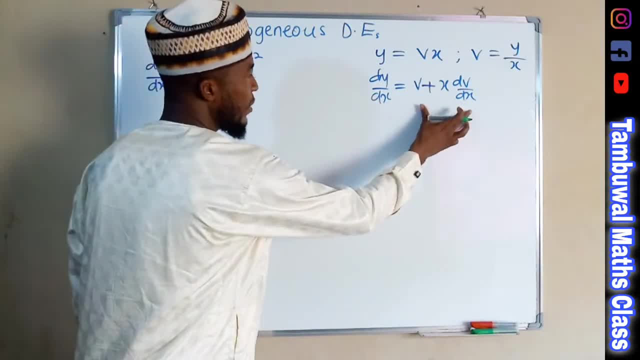 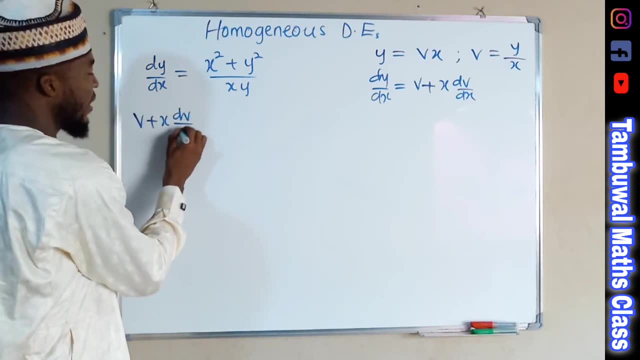 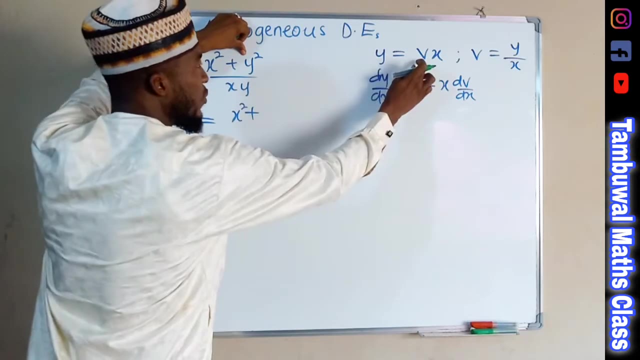 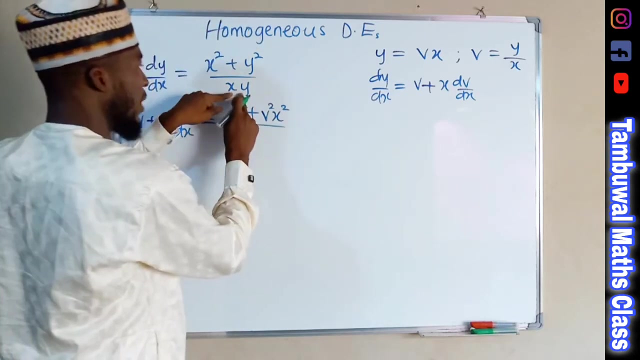 So we have dy over dx here, which is equal to v, plus x, dv over dx. And to the right hand side we have x squared plus this is y squared, but y equal to vx. So we have v squared, x squared. Divide by, we have x multiplied by y. 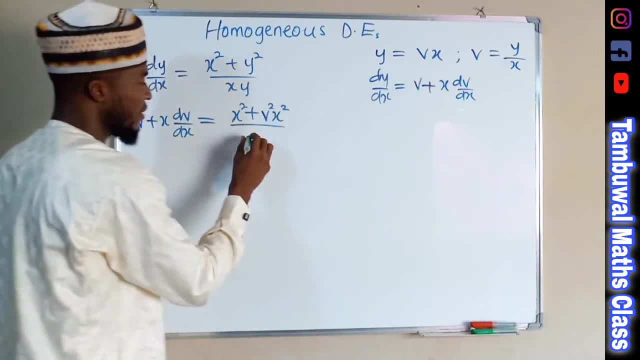 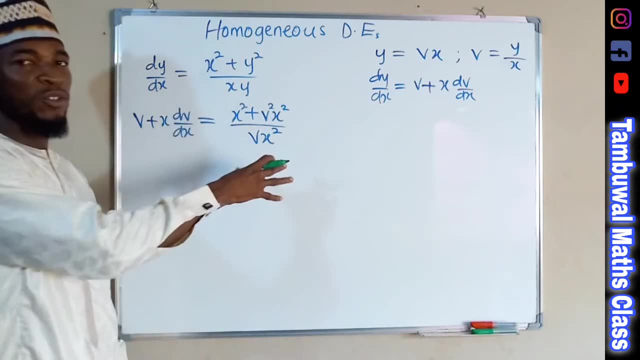 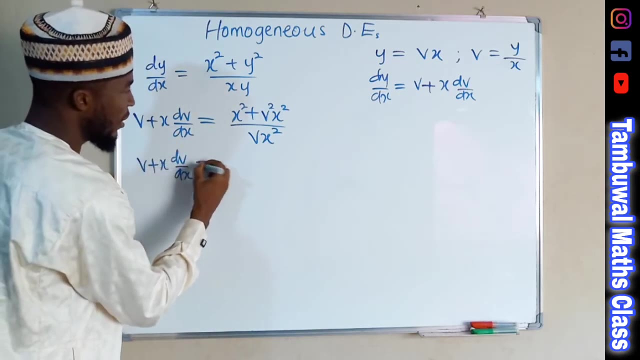 This is the same thing as saying x times vx, which is the same thing as vx squared Each time now contains x squared, which you can divide Each time by x squared to clear that. So we have v plus x. dv over dx equals x squared divided by x squared is 1.. 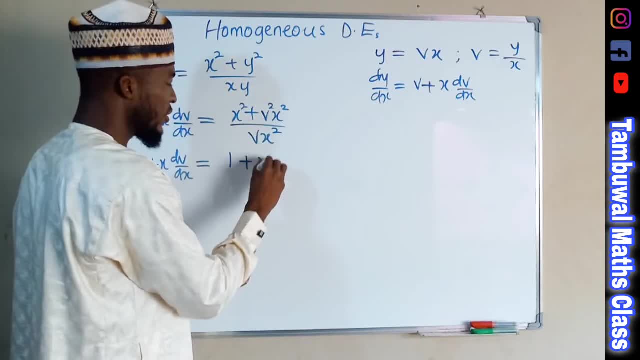 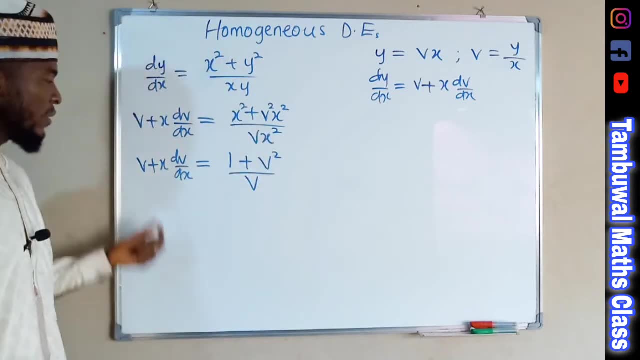 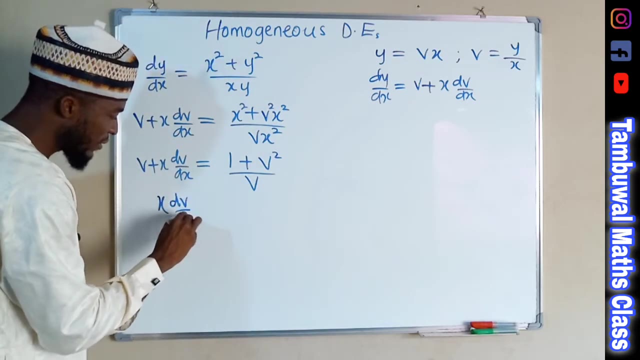 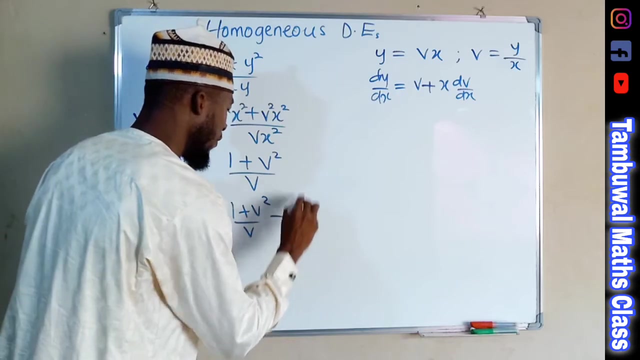 Plus v squared. x squared. divided by x squared is just v squared This time, divided by x squared is v. Still, we have v here, which we want to now take to the right hand side, Leaving x dv over dx. This is equal to 1 plus v squared over v minus v. 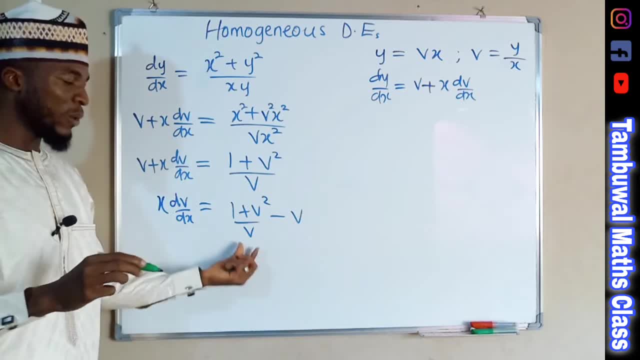 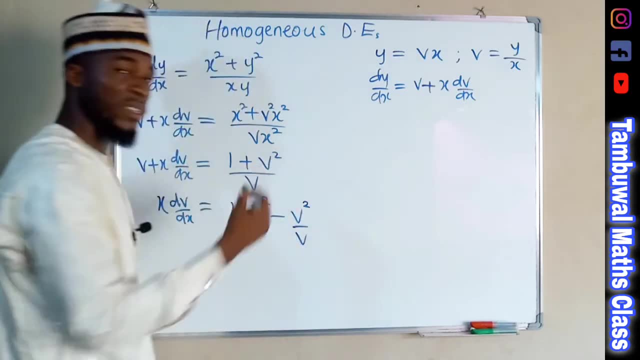 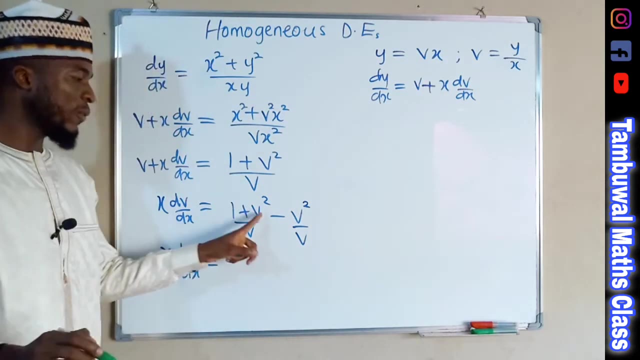 But you can write this in rational form. in such a way they will have a common denominator: By multiplying top and the bottom by v, So that we have v squared divided by v, which is the same thing as v, x. dv over dx is now equal to v squared minus v squared is 0, leaving only 1.. 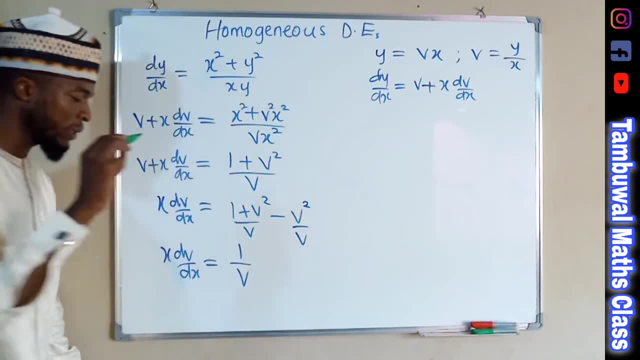 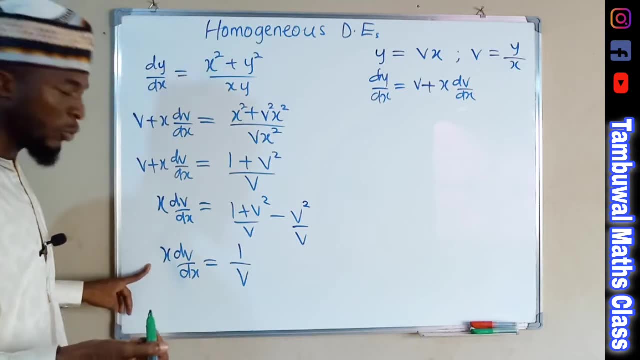 And common denominator. we have v. Now we want to separate the variables. A. v is dividing here. Once it crosses over, it will multiply. So we have v Already. we have dv here. dv. We want to take x to the right hand side. 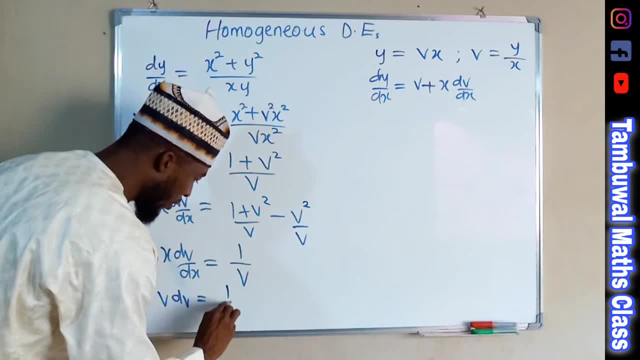 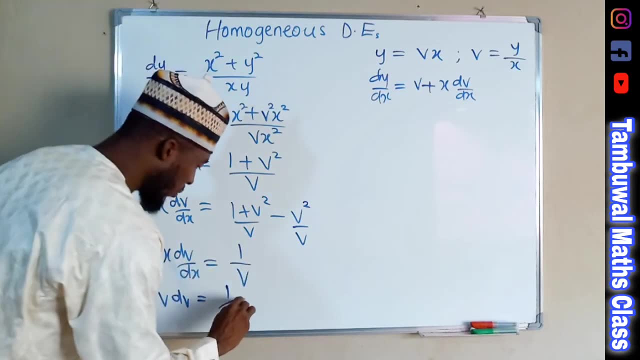 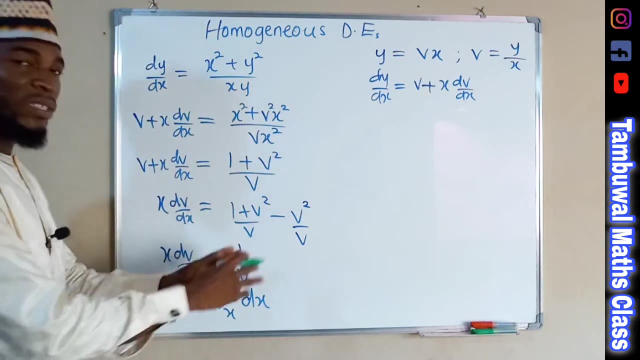 It is multiplying here. To the right hand side it will divide. So we have 1 over x. Again we have dx. It is dividing here. Once it crosses over, it will multiply. Now we have separated the variables. What we are going to do left is to integrate both sides to obtain the solution. 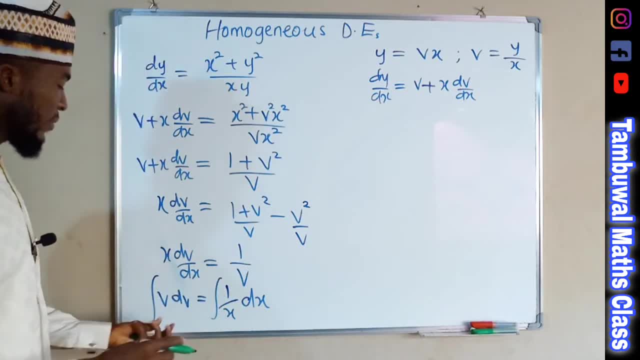 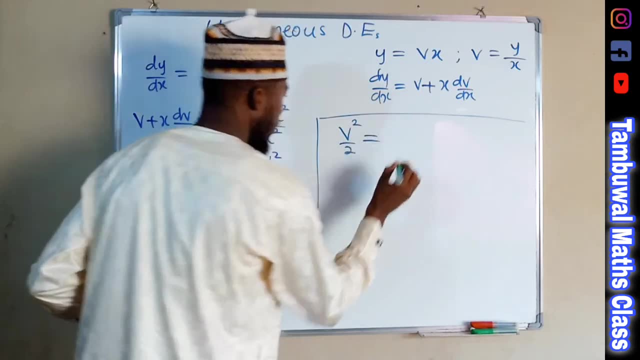 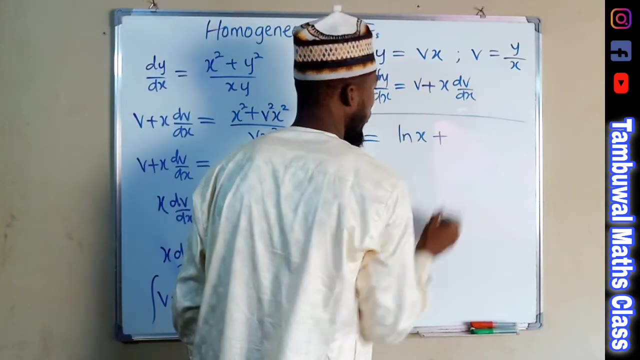 Integrate this side. Integrate this side. If you integrate v, you are going to obtain v squared over 2.. And to the right hand side, if you integrate 1 over x, you are going to obtain natural log of x Plus the constant of integration c. 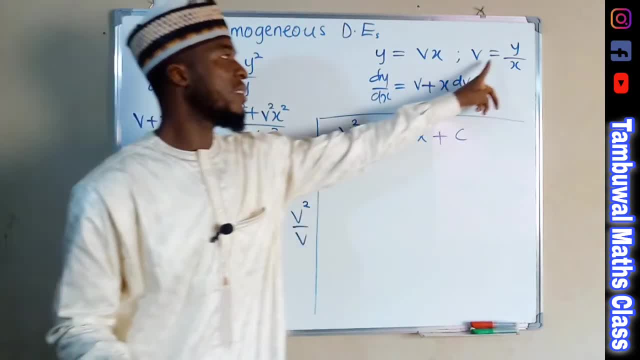 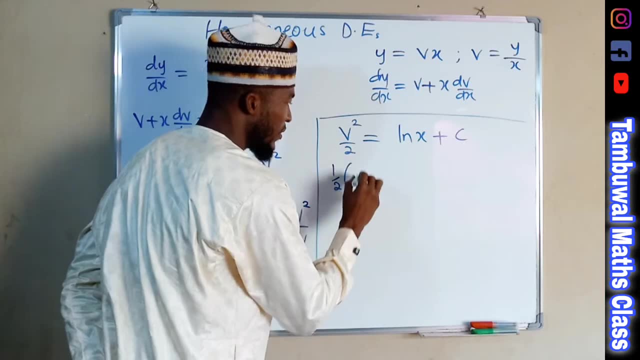 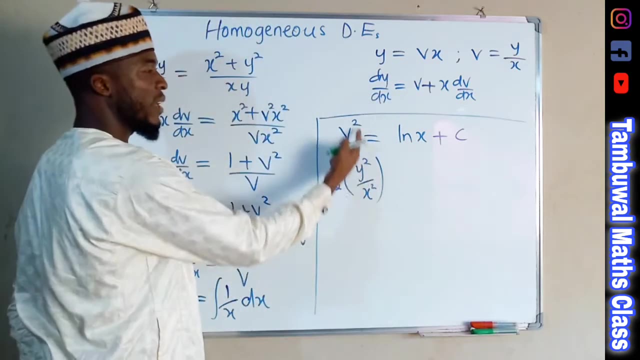 But we are not done yet, because v is equal to y over x, So we are going to replace this with y over x, So we have 1 over 2 outside, And inside we have y squared over x squared, because v is halving squared. 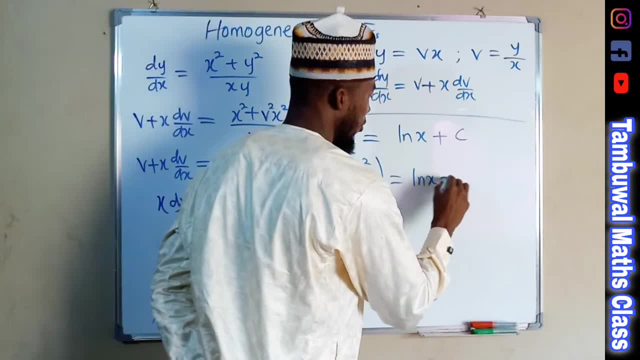 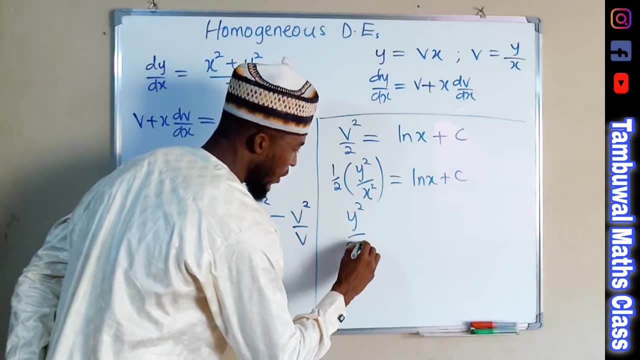 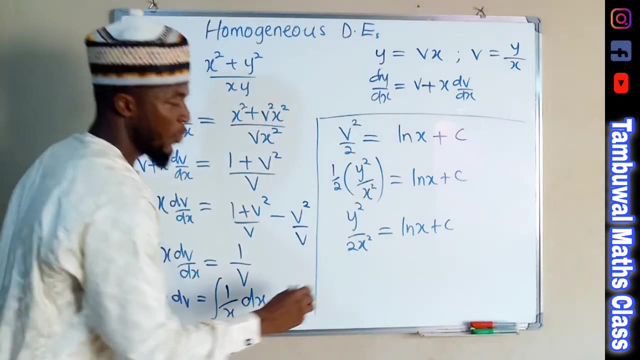 To the right hand side, we have natural log of x plus c. This is the same thing as y squared over 2x squared. This is equal to natural log of x plus c- y squared, if you multiply both sides by 2x squared. 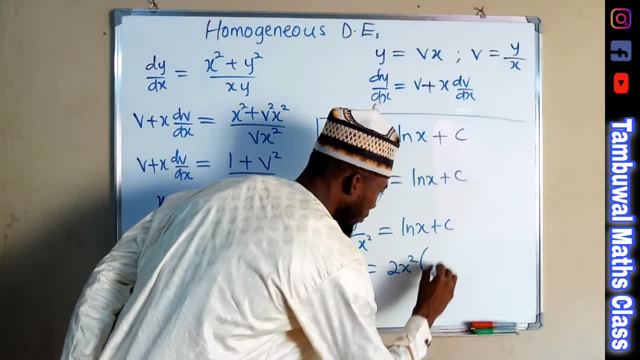 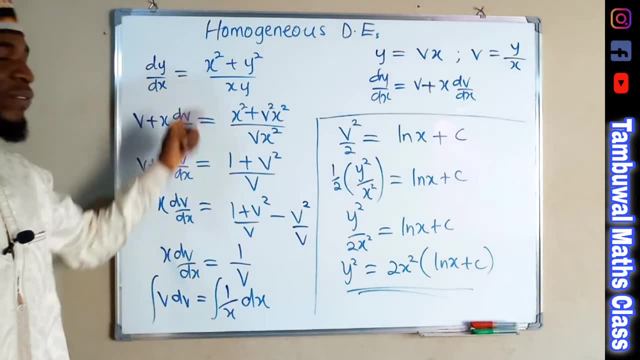 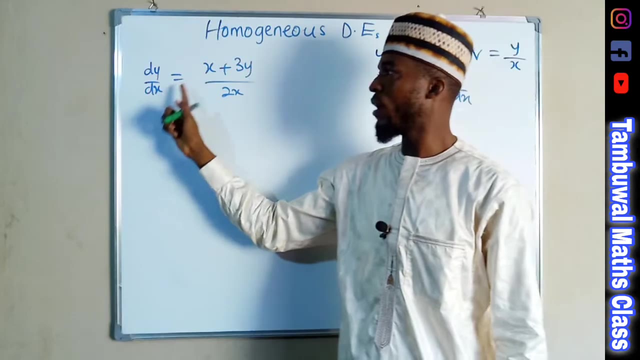 You are going to obtain 2x squared times the natural log of x plus c. Hence, this is the solution for this differential equation. Now let us look onto the next one. Here is our next problem. We have dy over dx to be equal to x, plus 3y over 2x. 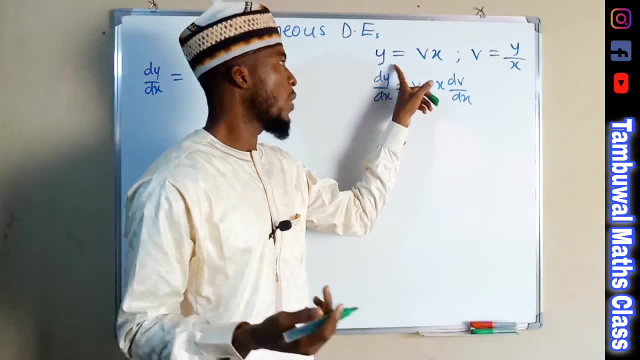 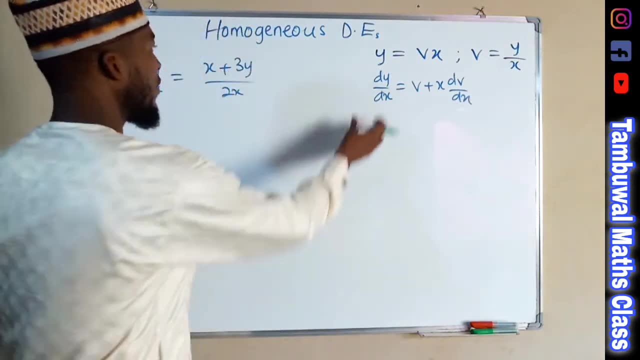 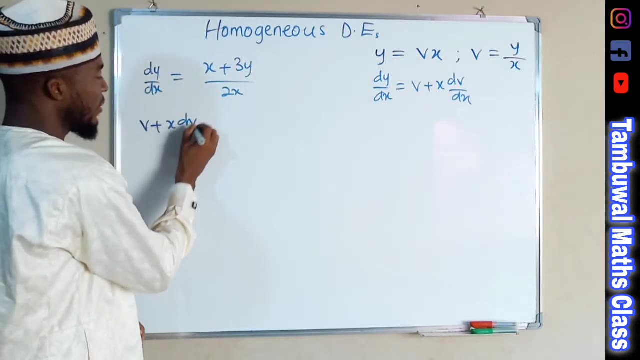 We are going to apply the same principle: y equal to vx, v equal to y over x, dy over dx is equal to this. We are going to replace dy over dx with this times, So we have v plus x, dv over dx. 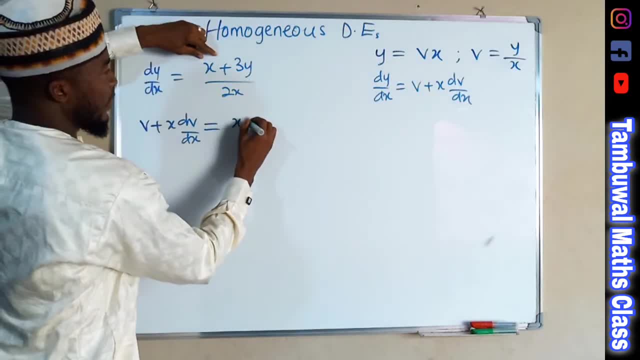 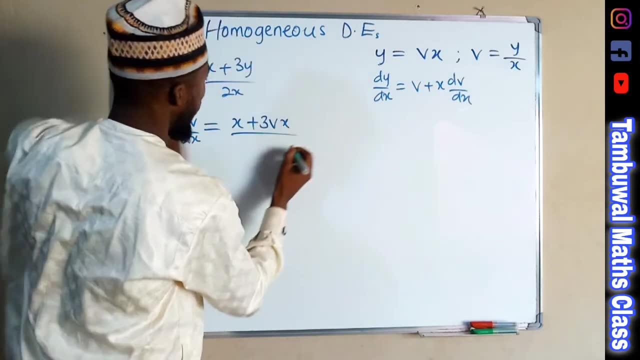 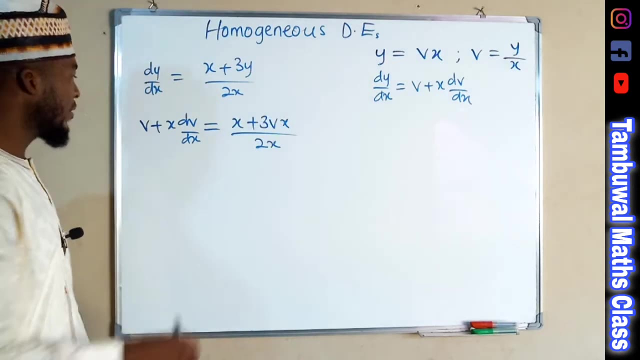 This is equal to: We have x plus 3 times y, 3 times this term. We have 3vx over 2x. Each term contains x. We are going to divide each term by x So that we have v plus x. dv over dx to the left hand side. 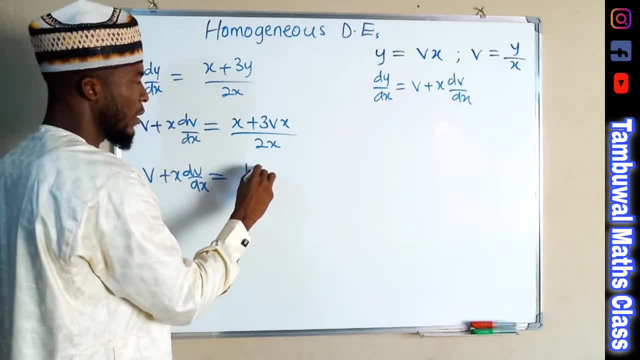 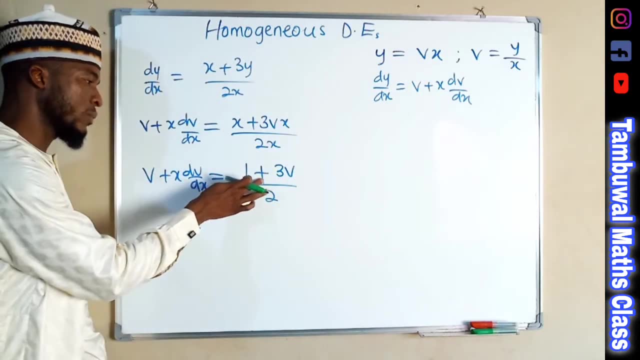 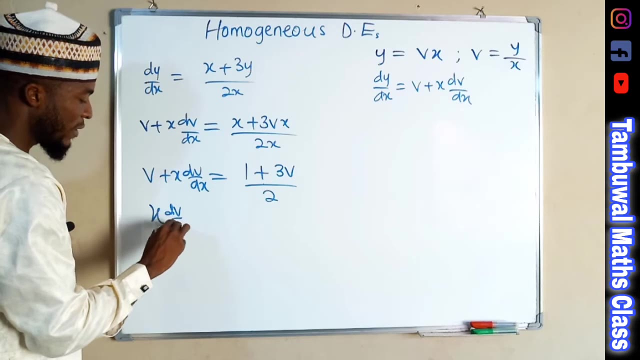 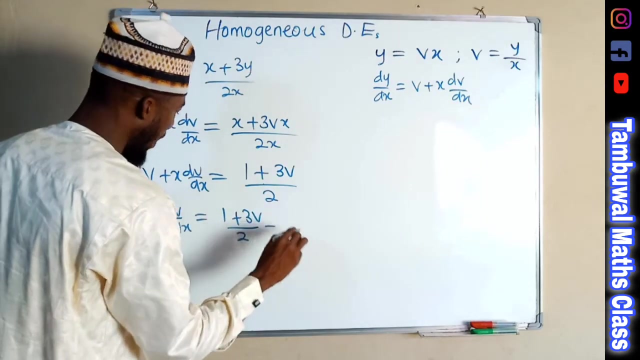 And to the right hand side, we have x divided by x is 1.. Plus this divided by x, We have 3v Over 2.. We have v here. We are going to subtract it from both sides. So we have x. dv over dx equals 1 plus 3v over 2 minus v. 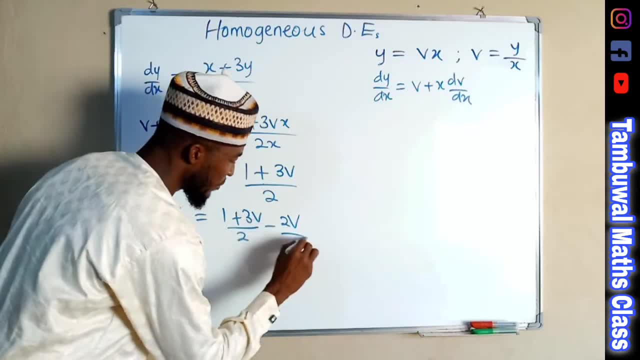 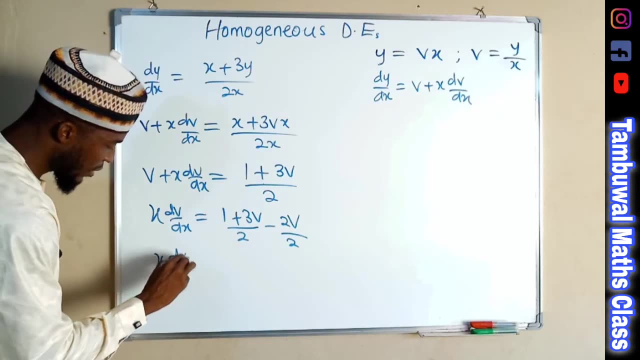 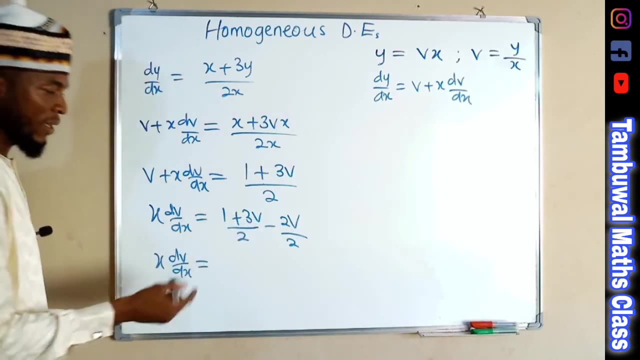 But you can write this v as 2v over 2. Such that we have common denominator x, dv over dx. dv over dx Is now equal to This minus. this is v. So we have 1 plus v over the common denominator 2.. 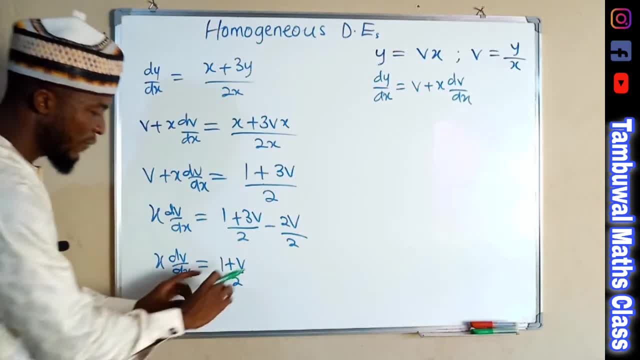 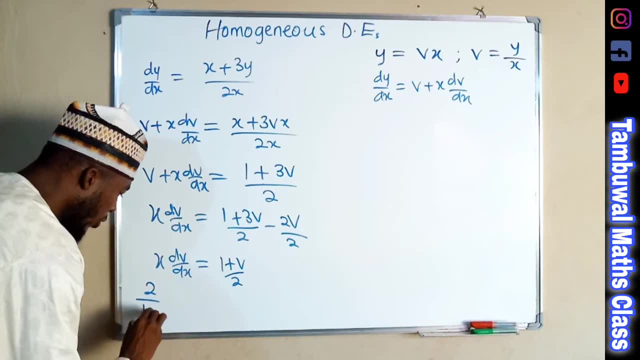 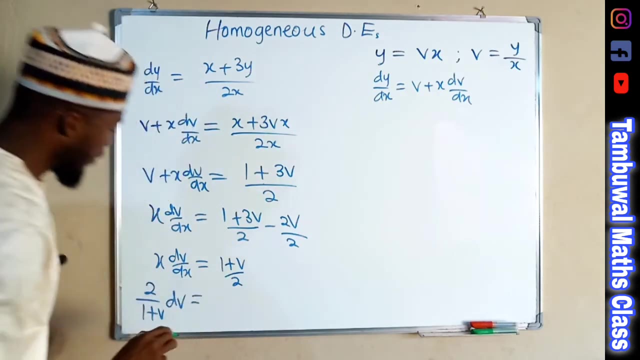 Now we are free to separate the variables. If you multiply both sides by the reciprocal of this, You are going to obtain 2 over 1 plus v. So we have dv here And to the right hand side. this is multiplying. It will divide. 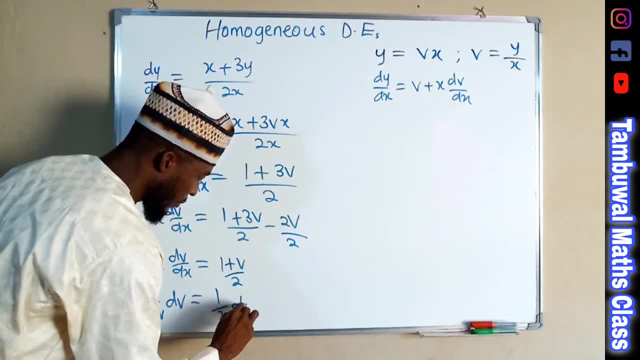 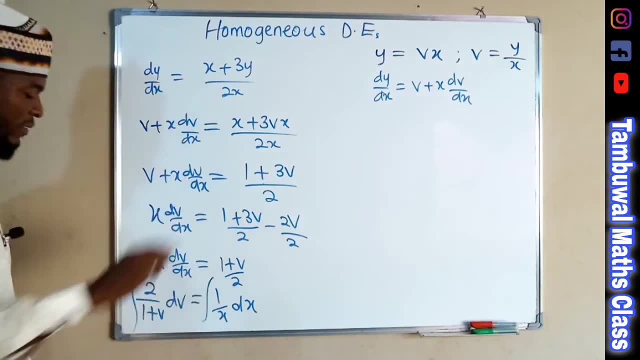 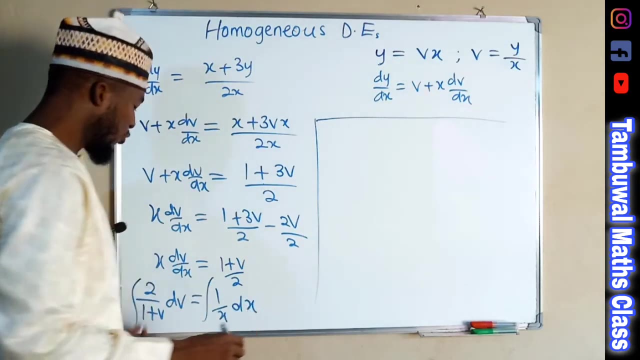 dx is dividing, It will multiply. Next step: Integrate both sides. Integrate this side, Integrate the other side. You can factor out 2 so that you have 1 over 1 plus v left. If you integrate it, you are going to obtain the natural log of 1 plus v. 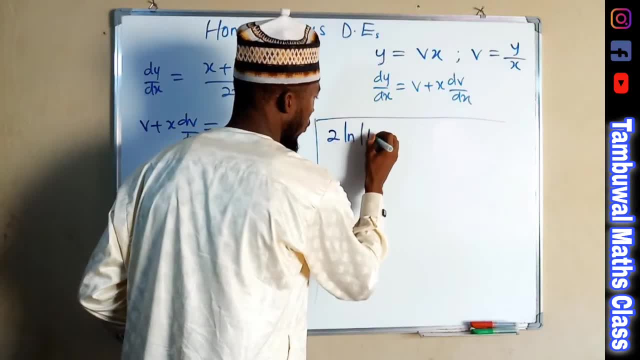 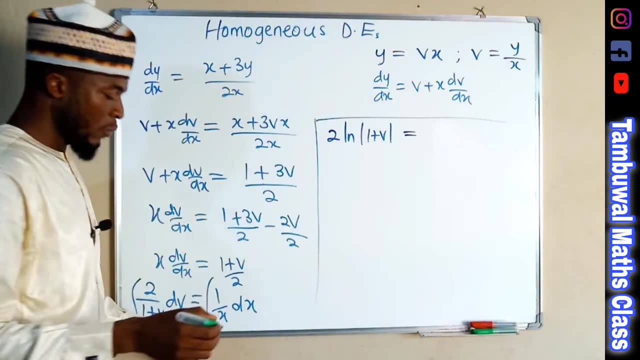 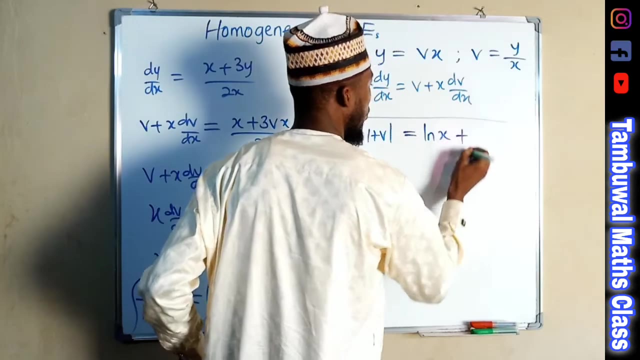 So we have 2 outside Natural log of 1 plus v. In absolute form This is equal to 1 over x. if you integrate it, you obtain Natural log of x Plus the constant of integration, which you can also write in log form.